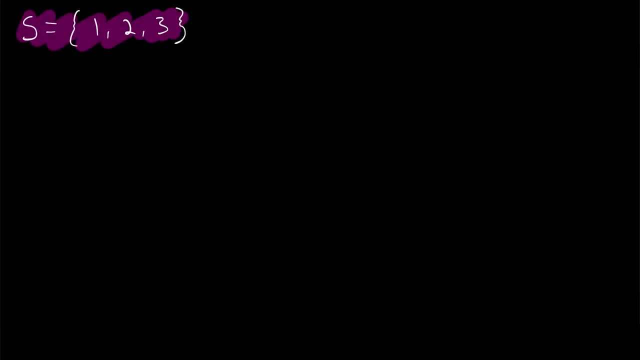 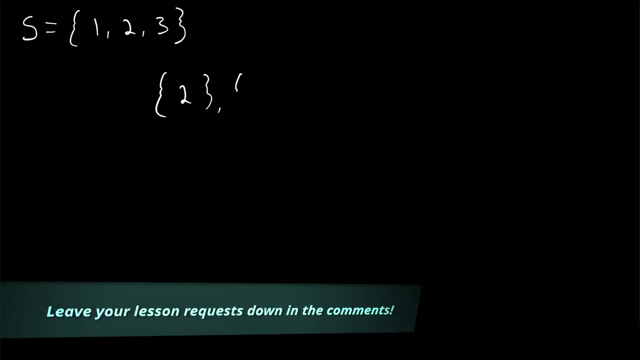 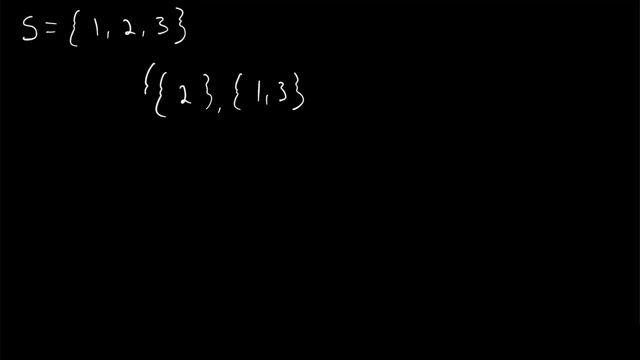 Here we've got a set called S. Imagine if we wanted to separate S into two parts. We could separate it into its even elements and into its odd elements, 1 and 3.. Then if we put these two subsets of S into a set all on their own, we could call this set P, and that is a partition of the. 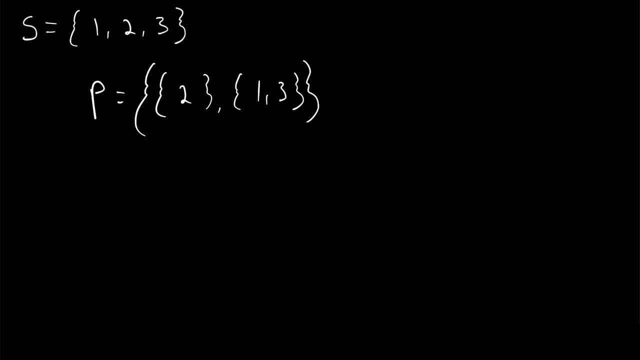 set S. In today's Wrath of Math lesson we'll be going over the definition of partitions of a set and we'll see some more examples. Partitions of a set is a pretty common concept in math, so it's definitely a useful term to be familiar with. Let's take a closer look at our partition P. 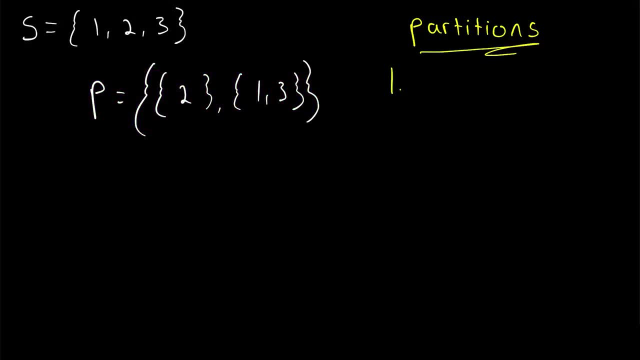 Why is this a partition of S? Firstly, P is a partition of S because it is a collection of non-empty subsets of S. When we're talking about partitions, of course we're separating a set into different parts and we're not particularly 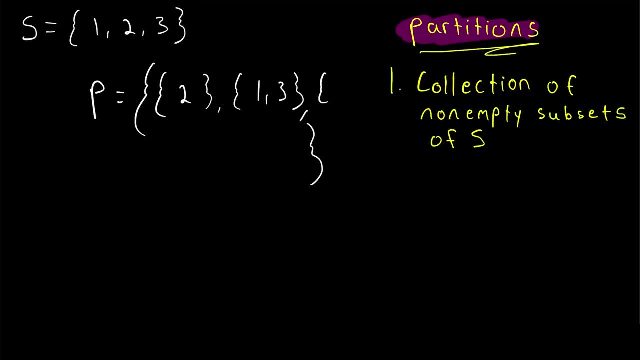 interested in, one of those parts being the empty set. So a partition is not allowed to contain the empty set. And also, of course, since P is a partition of S, all of the sets in P must be subsets of S. If we're separating S into parts to form a partition, of course each part must. 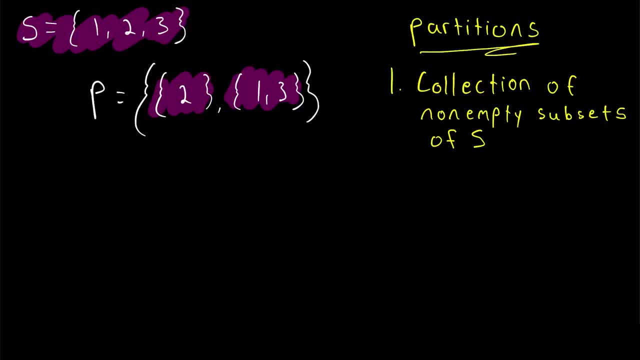 only contain elements of S. They've got to be subsets of S, And then the only second thing necessary for this to be a partition of S is to separate S into parts. So if we're separating S is that every element of S has to be in exactly one element of P And, of course, the partition P. 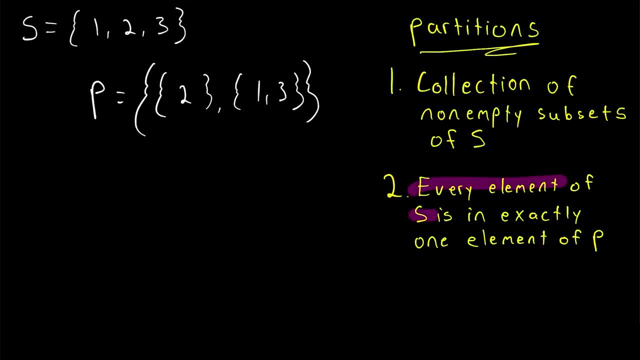 is made of subsets of S, So every element of S must be in exactly one of the subsets that are contained in P. So the two important points about this restriction are that every element of S is included in some part of the partition and no elements of S are included in. 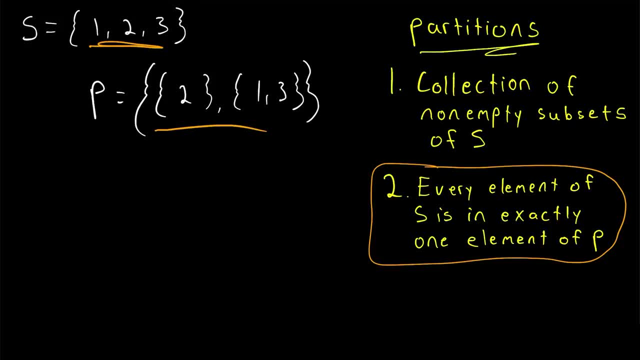 more than one part of the partition. So we are separating S into these disjoint parts. All right, I think it's time for some more examples. Is this a partition of our set? S It is not, because it contains the empty set, and a partition has to only contain non-empty subsets. 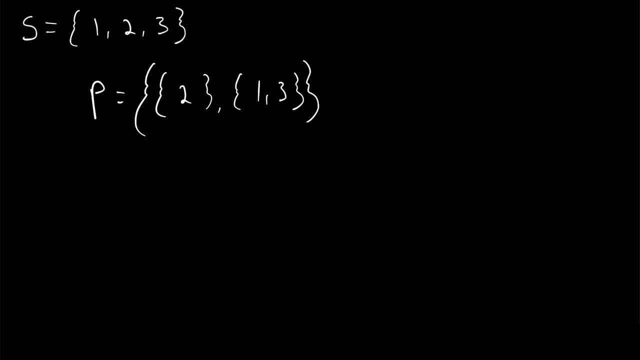 set S. In today's Wrath of Math lesson we'll be going over the definition of partitions of a set and we'll see some more examples. Partitions of a set is a pretty common concept in math, so it's definitely a useful term to be familiar with. Let's take a closer look at our partition P. 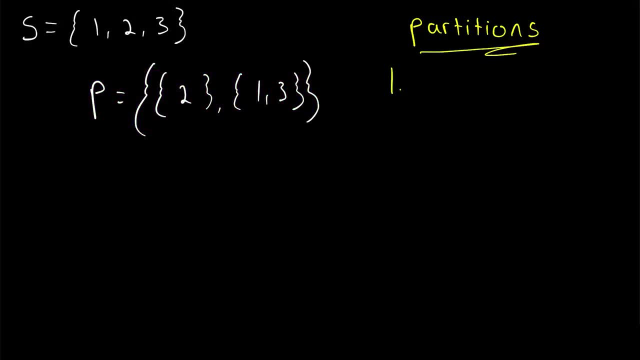 Why is this a partition of S? Firstly, P is a partition of S because it is a collection of non-empty subsets of S. When we're talking about partitions, of course we're separating a set into different parts and we're not particularly 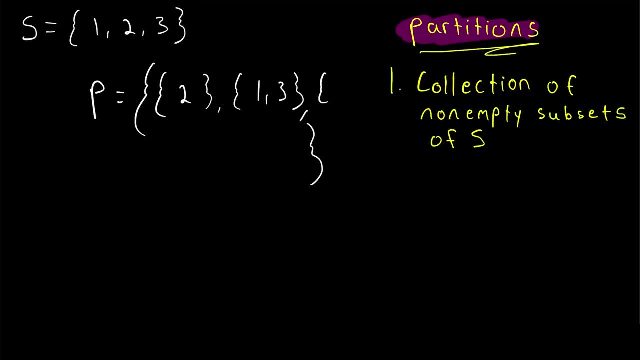 interested in, one of those parts being the empty set. So a partition is not allowed to contain the empty set. And also, of course, since P is a partition of S, all of the sets in P must be subsets of S. If we're separating S into parts to form a partition, of course each part must. 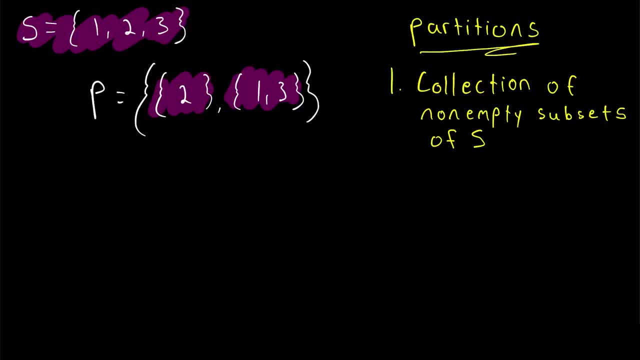 only contain elements of S. They've got to be subsets of S, And then the only second thing necessary for this to be a partition of S is to separate S into parts. So if we're separating S is that every element of S has to be in exactly one element of P And, of course, the partition P. 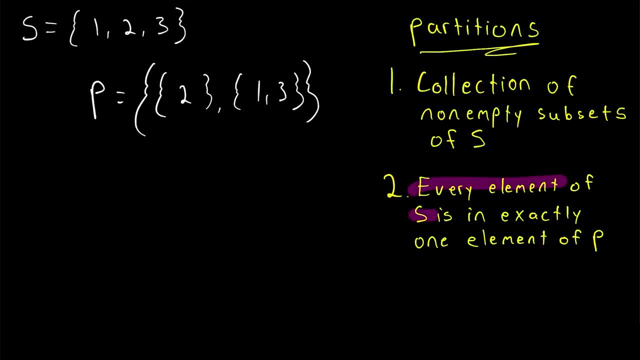 is made of subsets of S, So every element of S must be in exactly one of the subsets that are contained in P. So the two important points about this restriction are that every element of S is included in some part of the partition and no elements of S are included in. 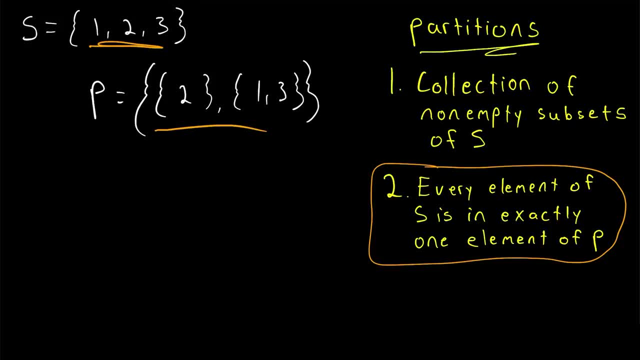 more than one part of the partition. So we are separating S into these disjoint parts. All right, I think it's time for some more examples. Is this a partition of our set? S It is not, because it contains the empty set, and a partition has to only contain non-empty subsets. 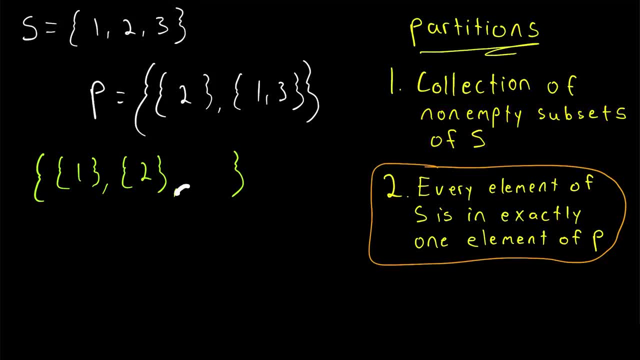 of the partitioned set. All right, so what if we fix that problem and get rid of the empty set? Is this a partition of S? now, It is a partition because of the second condition, that every element of S has to be in exactly one. 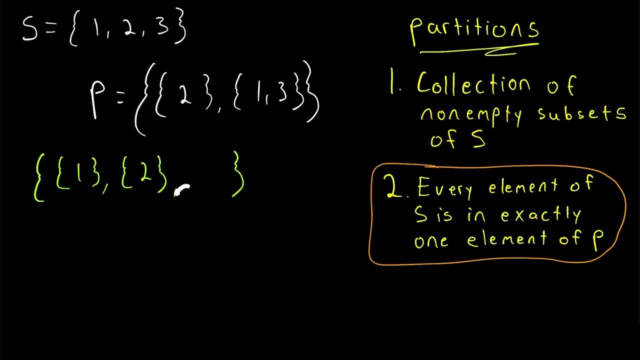 of the partitioned set. All right, so what if we fix that problem and get rid of the empty set? Is this a partition of S now? No, it's still a partition because of the second condition, that every element of S has to be in exactly one element of our partition. 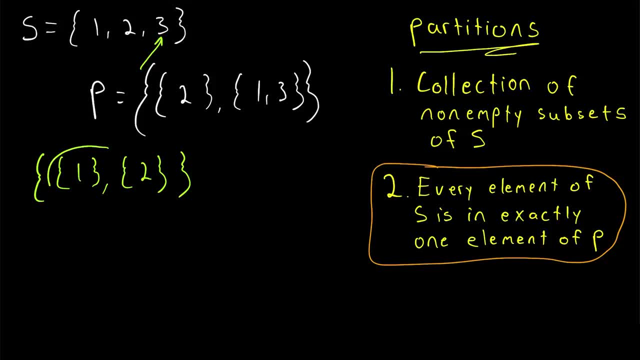 We see that the element 3 in S is not in any of the elements of this set. so this green set is not a partition. All right, so what if we go ahead and fix that problem and put the element 3 that we were missing in both parts of this set? 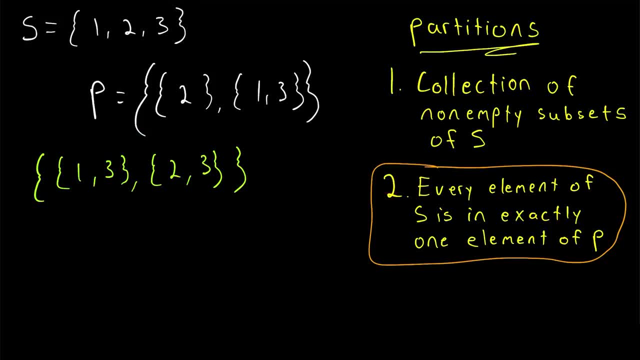 Now, is this a partition? Still no, It's still vital, violating the second condition. While every element of s is now in one of the parts of this set, the element 3 is in two parts of the set. But in order for it to be a partition, 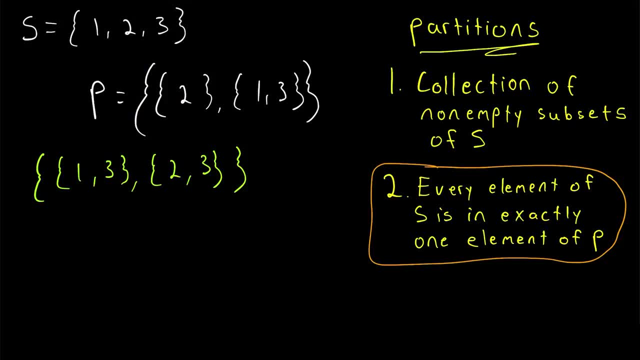 every element of s needs to be in exactly one part of the partition. So if we go ahead and erase 3 from that element of the set, now we've got a partition of the set s And in fact this is the exact same partition we have here. This is the partition p. 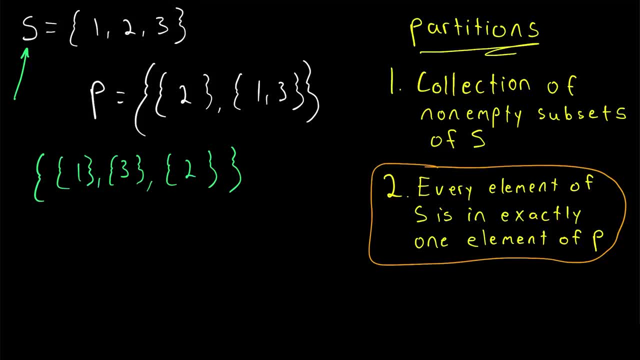 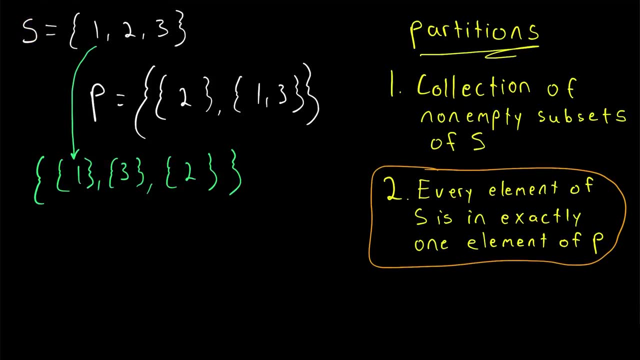 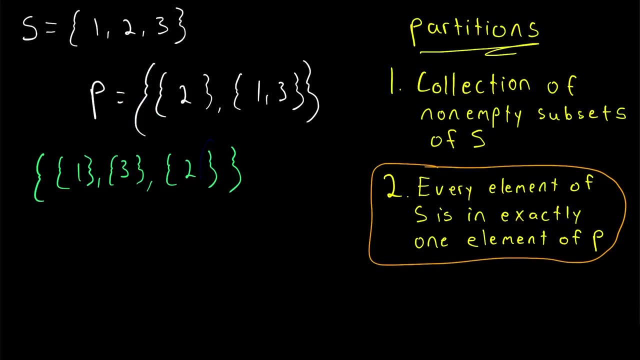 All right, how about this set? Is this set a partition of s? Yes, indeed it is. It contains only non-empty subsets of s, and every element of s is in exactly one of the elements of the partition. So this is a valid partition of s. What if we slightly changed this partition? so 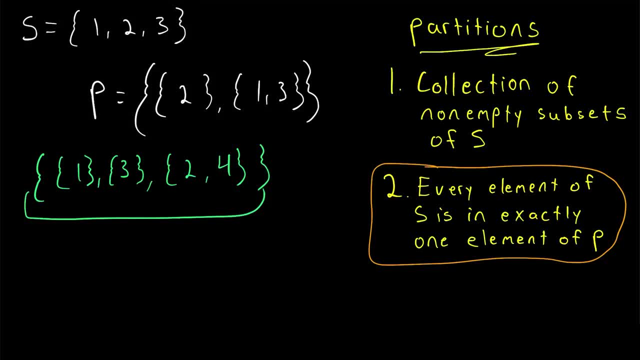 that it looked like this: This is no longer a partition, because it's not a collection of subsets of s, because the set containing 2 and 4 is not a subset of s, because the element 4 is not in s. Now, how about this? What if we just take the set s itself and put that in another set? 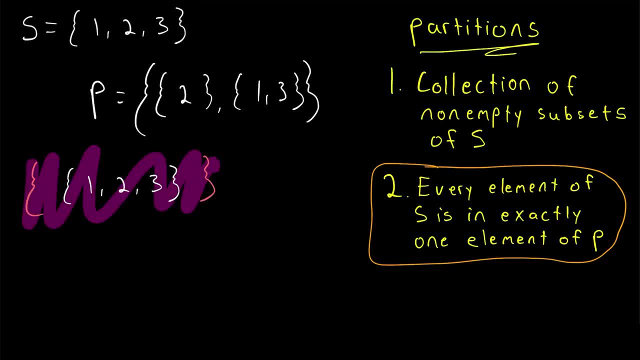 Does that form a partition? Yes, indeed, this is a partition of s, because it's a collection of non-empty subsets of s, since every set is a subset of itself and every element of s is in exactly one of the subsets contained in the partition. They all happen to be in the same set. 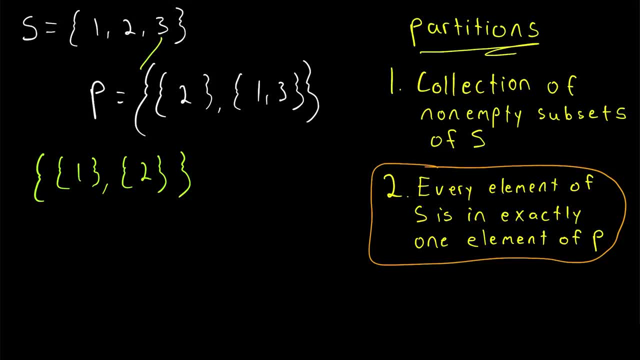 element of our partition. We see that the element three in S is not in any of the elements of this set. so this green set is not a partition. All right, so what if we go ahead and fix that problem and put the element three that we were missing in both parts of this set? Now is this a partition? 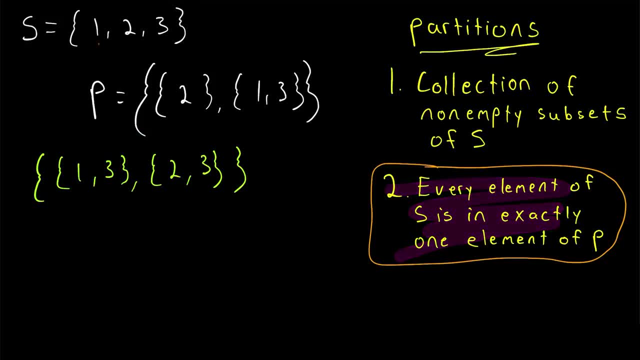 Still no, violating the second condition. While every element of s is now in one of the parts of this set, the element 3 is in two parts of the set, But in order for it to be a partition, every element of s needs to be in exactly one part of the partition. So if we go ahead and erase 3, 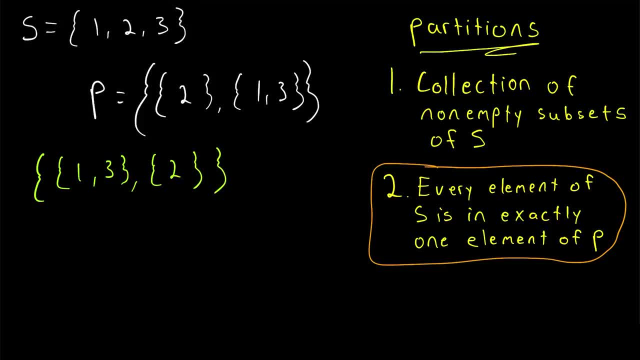 from that element of the set. now we've got a partition of the set s And in fact, this is the exact same partition we have here. This is the partition p. All right, how about this set? Is this set a partition of s? Yes, indeed, it is. It contains only non-empty subsets of s and every. 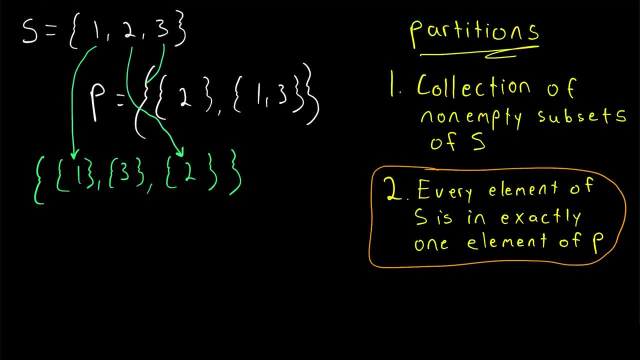 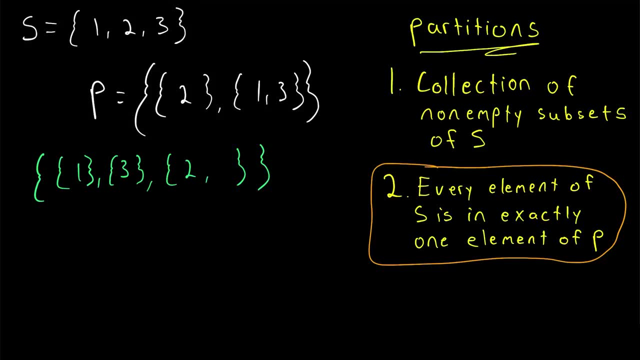 element of s is in exactly one of the elements of the partition, So this is a valid partition of s. What if we slightly changed this partition so that it looked like this: This is no longer a partition because it's not a collection of subsets. 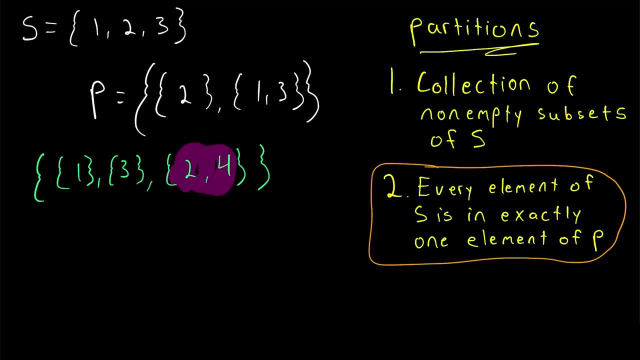 Because the set containing 2 and 4 is not a subset of s, because the element 4 is not in s. Now, how about this? What if we just take the set s itself and put that in another set? Does that form a partition? Yes, indeed, this is a partition of s, because it's a collection of non-empty. 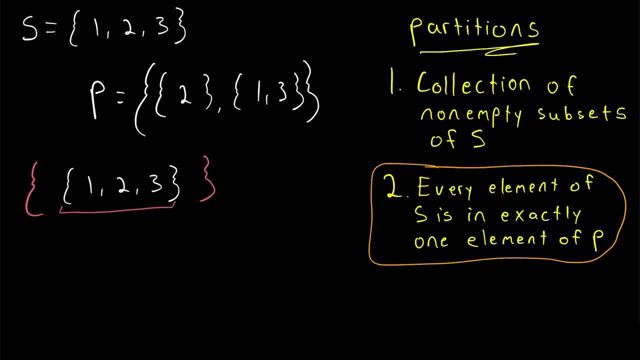 subsets of s, since every set is a subset of itself and every element of s is in exactly one of the elements of the partition. So this is a collection of non-empty subsets of s, exactly one of the subsets contained in the partition. They all happen to be in the same set. 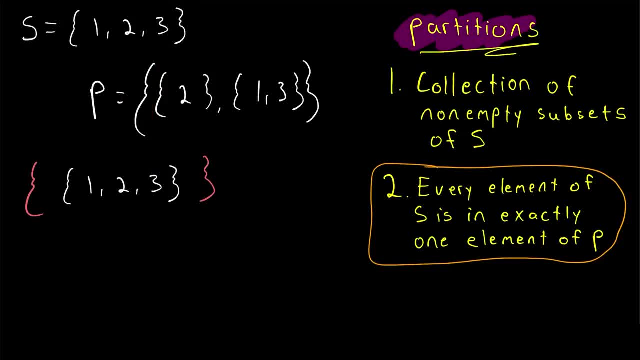 in the partition, but that's fine. So that's what a partition of a set is. To be clear about the language, remember that for a partition of a set s, the elements of the partition are subsets of that set s. So the set containing 2,, for example, is an element of our partition p and it's a. 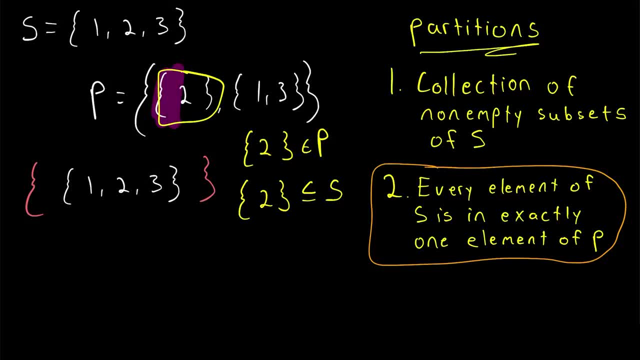 subset of that set s. So that's what a partition of a set is. To be clear about the language, remember that for a partition of a set s, the elements of the partition are subsets of that set s. To help avoid confusion, when talking about a partition, you might choose to call its elements. 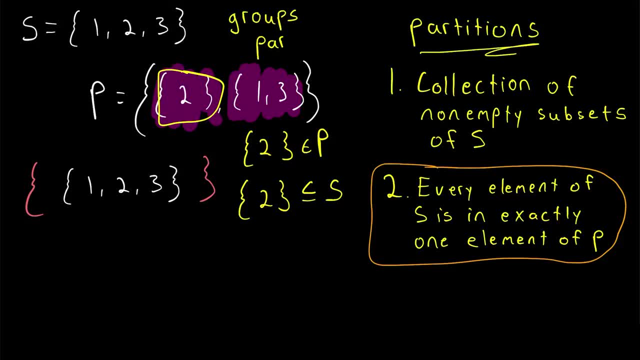 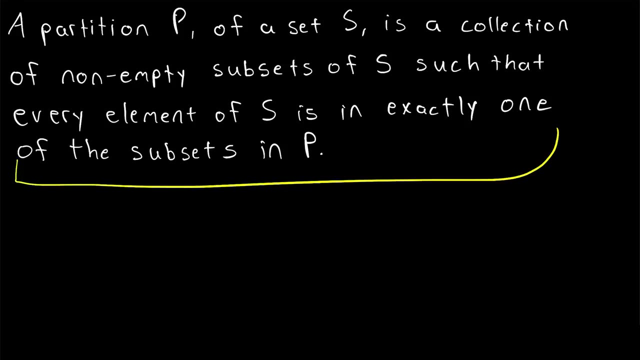 the groups of the partition, or maybe the parts of the partition. Then we might say that the partition p partitions the set s or separates the set s into two groups. Now for your reading and viewing pleasure, here is a more well-written definition. A partition p of a set s is a. collection of the set s. So that's what a partition of a set s is. So that's what a partition of a set s is. So that's how you laundry and hand提ins is. I think that's a really powerful definition of. 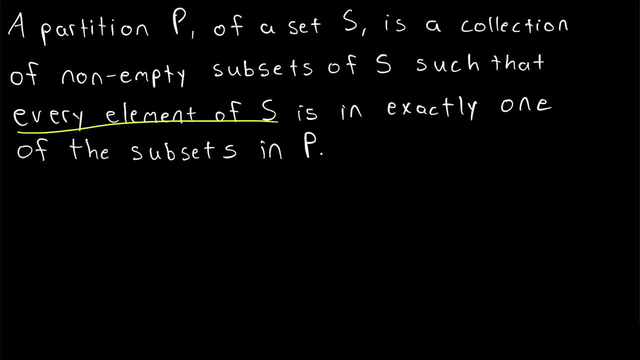 non-empty subsets of s, such that every element of s is in exactly one of the subsets in p. Remember: the subsets in p are elements of p. they are subsets of s, the set being partitioned. So the important thing to remember is that this says subsets in p, not subsets of p. 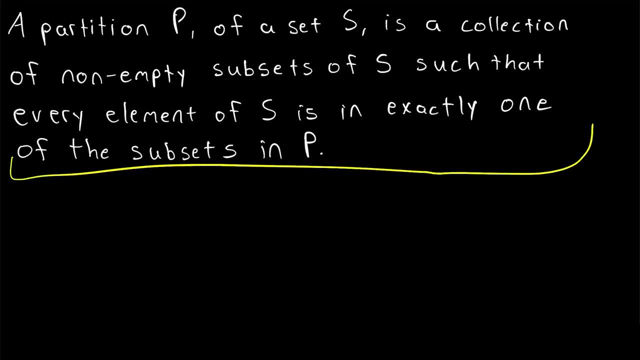 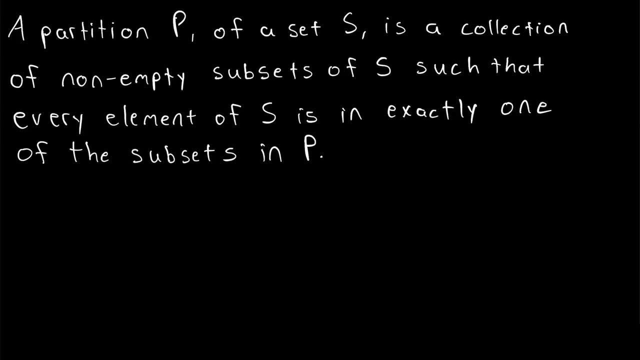 they are subsets of s. And notice: this definition is just exactly what we had above with the asked: brought 파. So this definition is just exactly what we had above with the asked: these two points just written in one nice concise definition. We could also represent a partition. 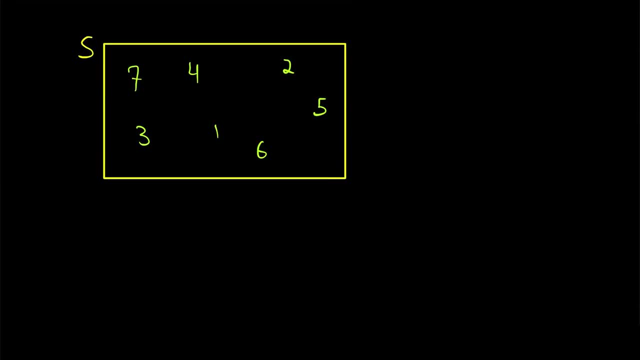 visually with a little diagram like this. This could be our set S and it contains these green elements. We could partition S into disjoint parts by drawing lines to create different groups in the set. The lines that I just drew define this partition. This drawing represents a collection. 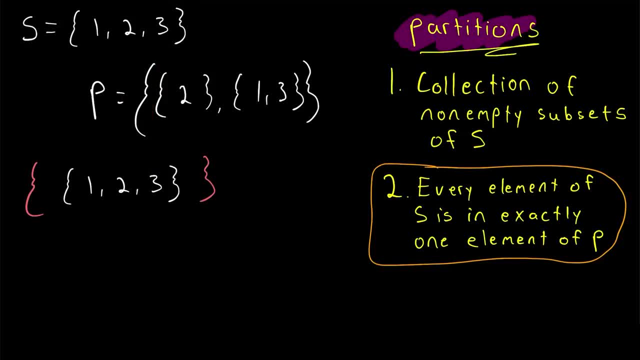 in the partition, but that's fine. So that's what a partition of a set is. To be clear about the language, remember that for a partition of a set s, the elements of the partition are subsets of that set s. So the set containing 2,, for example, is an element of our partition p and it's a subset. 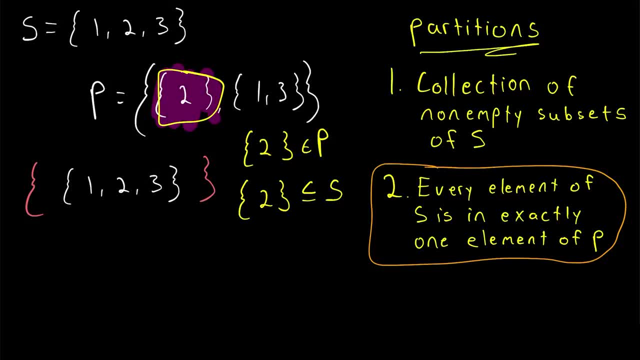 of our set s. To help avoid confusion when talking about a partition, you might choose to call its elements, the groups of the partition, or maybe the parts of the partition. Then we might say that the partition p partitions the set s or separates the set s into two groups. Now for your reading, and 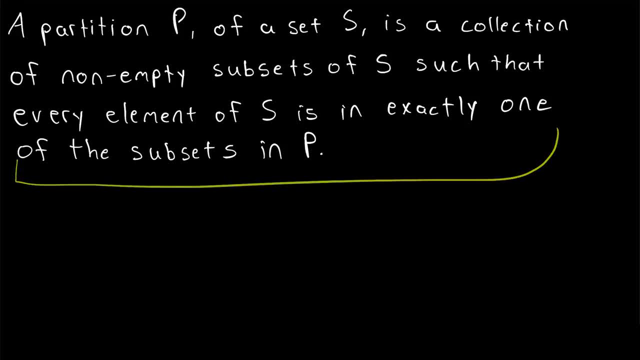 viewing pleasure. here is a more well-written definition: A partition p of a set s is a collection of non-empty subsets of s. So this is a collection of non-empty subsets of s, and it's a collection of non-empty subsets of s such that every element of s is in exactly one of the subsets. 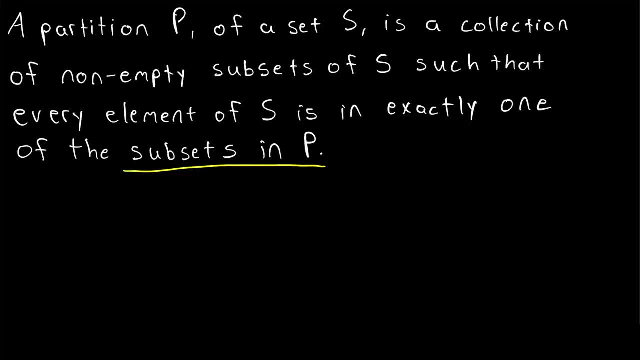 in p. Remember, the subsets in p are elements of p. they are subsets of s, the set being partitioned. So the important thing to remember is that this says subsets in p, not subsets of p. They are subsets of s. And notice, this definition is just exactly what we had above with. 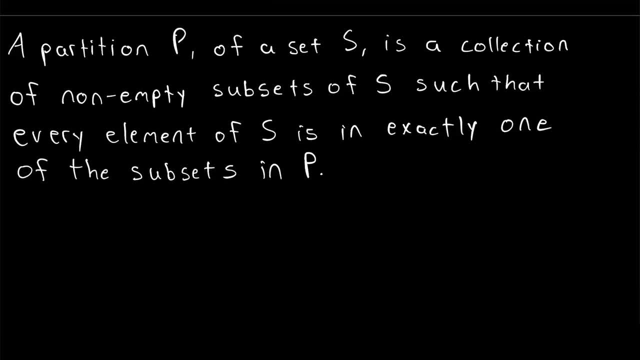 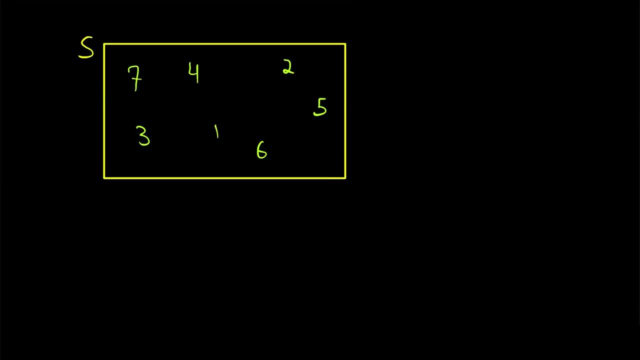 the elements of s being partitioned. So the important thing to remember is that this says these two points just written in one nice concise definition. We could also represent a partition visually with a little diagram like this: This could be our set s, and it contains these green 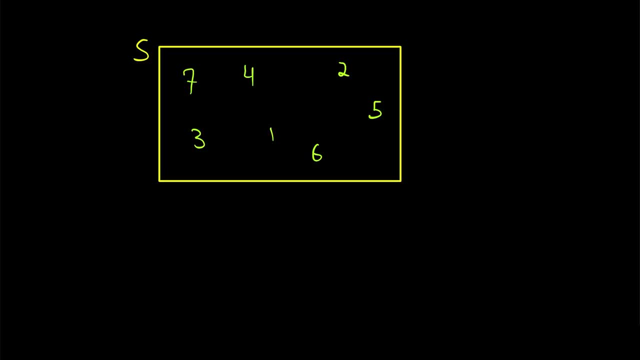 elements. We could partition s into disjoint parts by drawing lines to create different groups in the set. The lines that I just drew define this partition. This drawing represents a collection of non-empty subsets of s, So we could also represent a partition visually with a little diagram like. 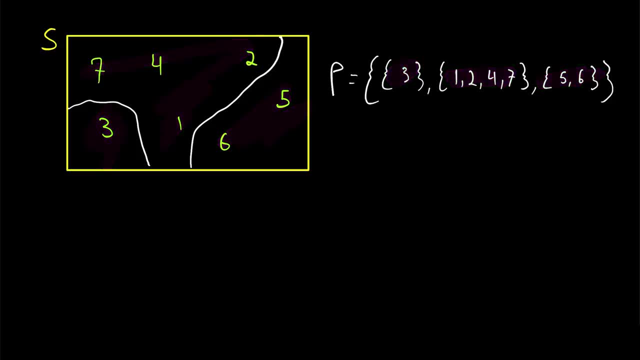 this. So the important thing to remember is that every element of s is in exactly one of these groups that we've separated them into, So no element is left out and no element is included in more than one group, And that's what a partition of a set is. A partition p of a set s.